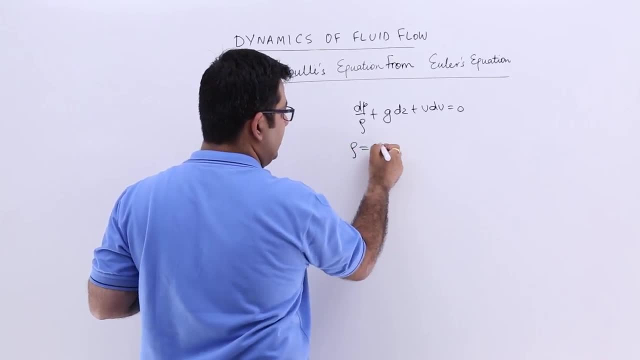 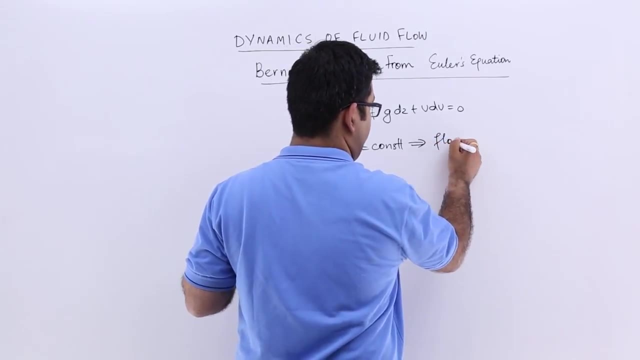 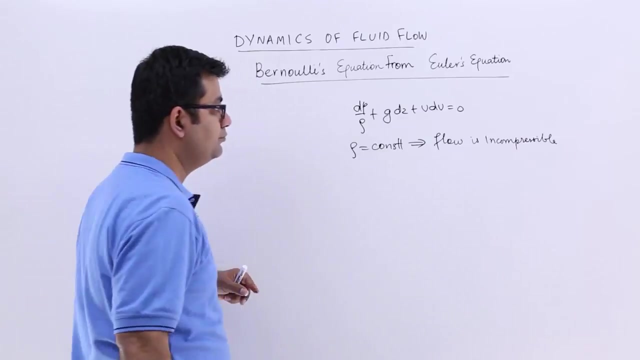 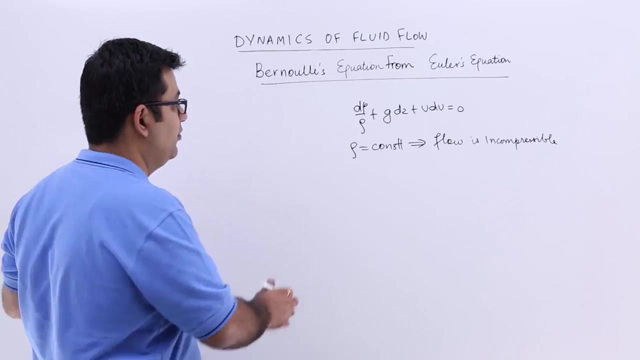 that for Bernoulli's equation we have to assume that the density is constant. This implies that the flow is incompressible. So you can derive the Bernoulli's equation with the help of this equation by integrating it. So when you integrate this equation, you get. 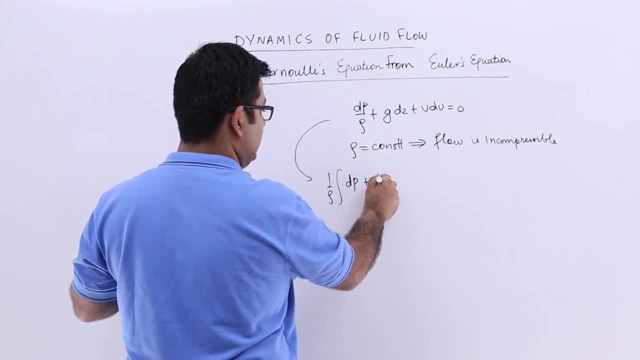 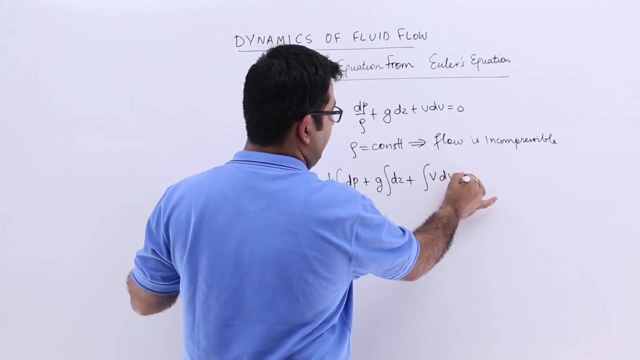 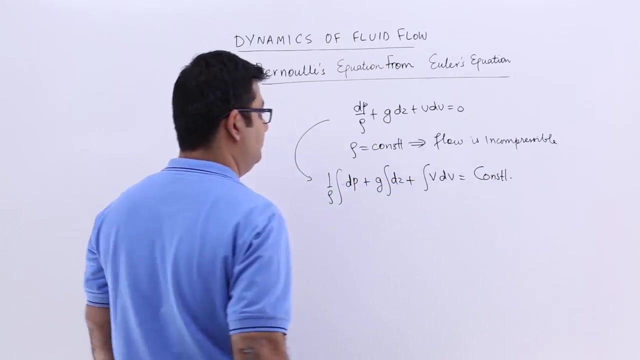 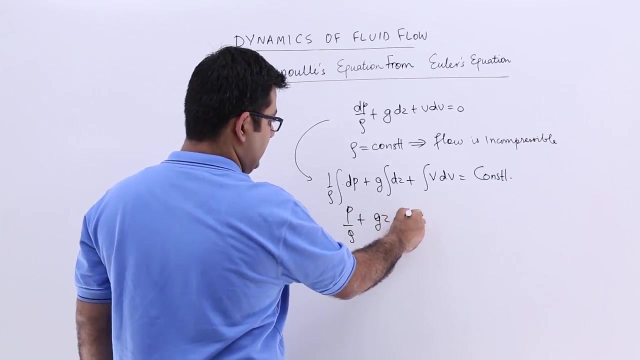 1 by rho, dp plus g is always a constant. You can have integral dz plus integral vdv is equal to a constant, because now 0 would become a constant value. okay, So this will become p upon rho plus g into z plus v. square upon 2g is equal to a constant. 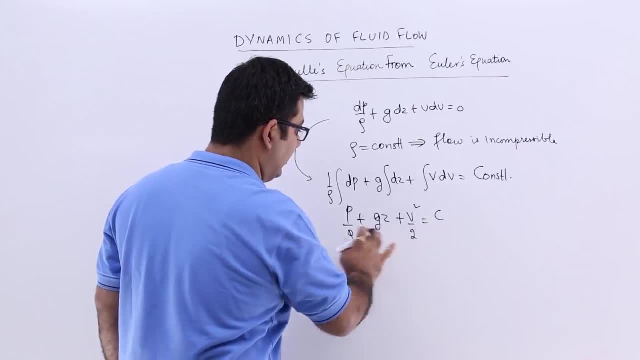 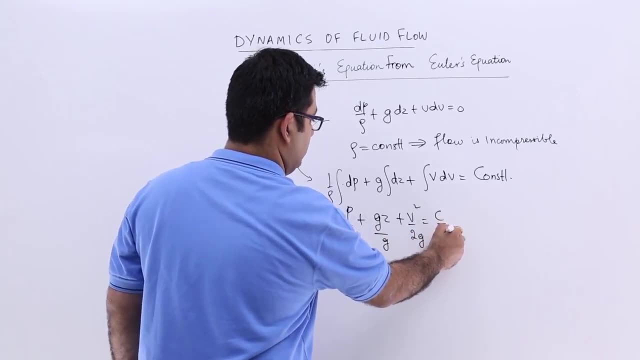 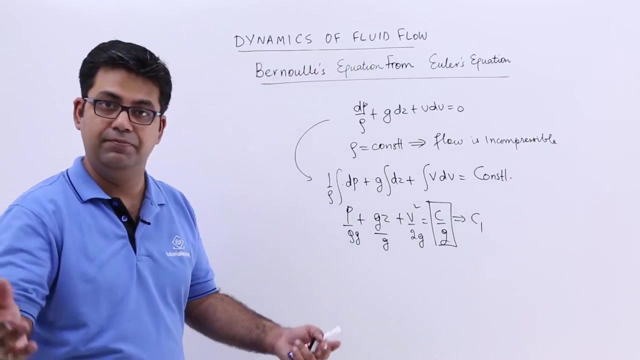 Now, this would only be 2 right now, So I will have to divide the entire equation by g. So this will become g by g by g, and this also divided by g. Now, this is constant upon constant. giving you another constant, Let us see one, Okay, So this will become p by rho, g plus. 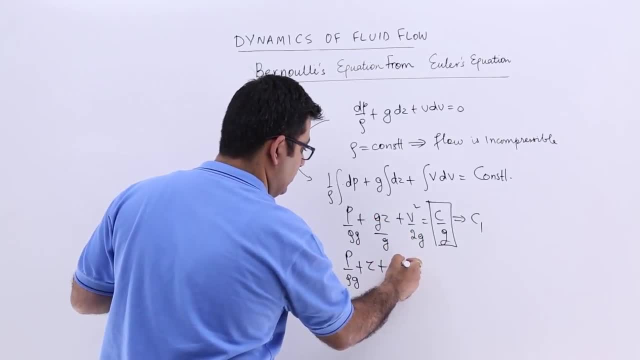 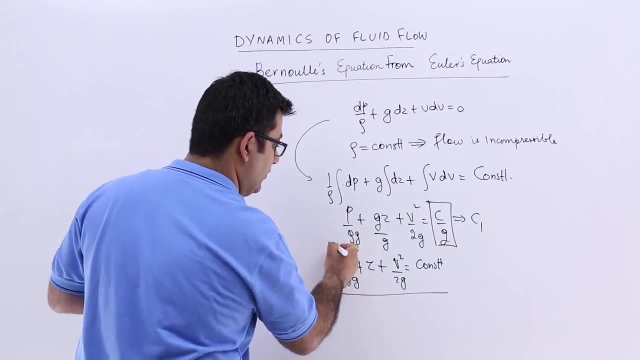 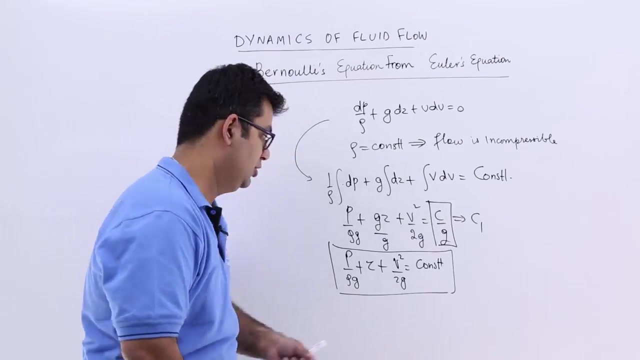 z plus v square upon 2g is equal to 0.. plus v square upon 2g is equal to constant. so this equation that you see, this is what we call the bernoulli's equation, and in this we have three terms. so you have the first. 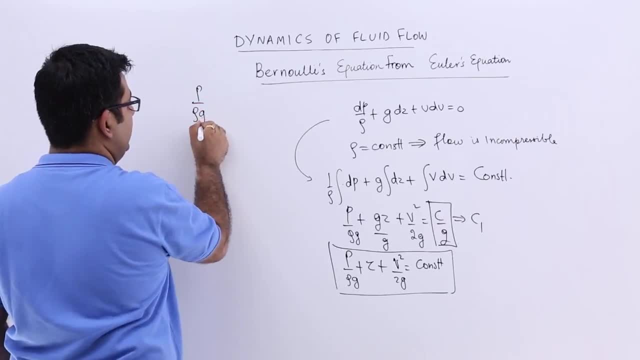 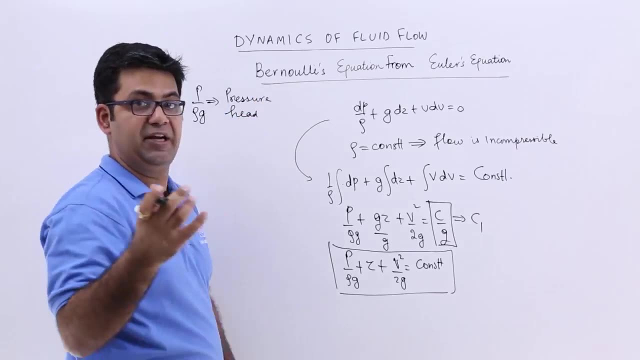 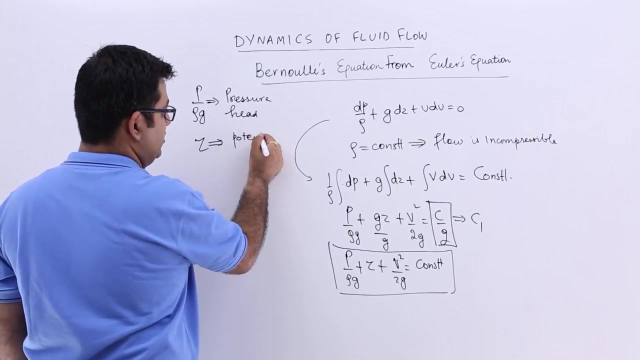 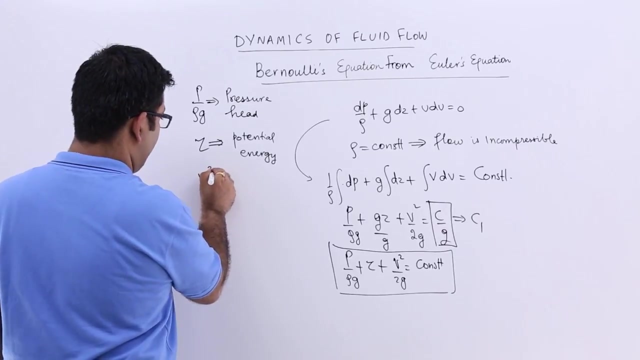 term, which is p by rho g, so p by rho g. this is called the pressure head, the pressure head or the pressure energy. then you have z, which is called the potential head or the potential energy. okay, and then we have v square upon 2g, which is called the velocity head or the. 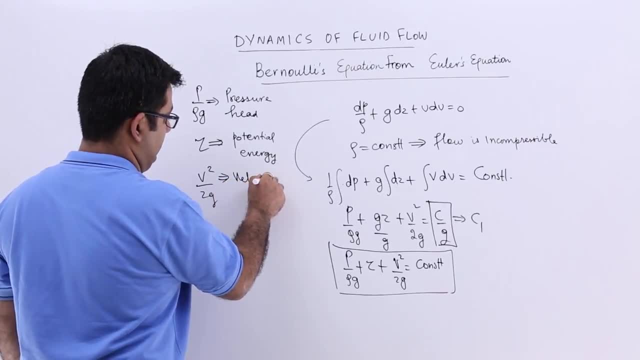 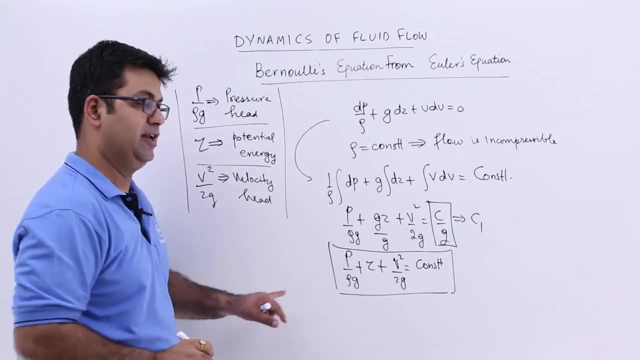 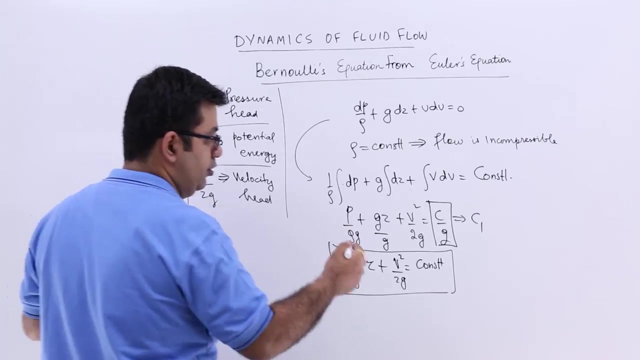 kinetic energy velocity head. alright, So this gives you the three terms. So this is the three terms that are there in the bernoulli's equation, which means that at any two points in a flow, let us say, if I draw a flow like this in a pipe, so this: